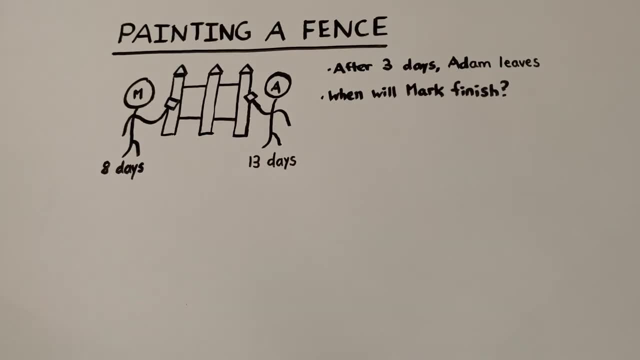 because then the remainder will be left for Mark on his own. So let's do that. Let's first find out how much of the fence Mark and Adam have painted together. So if Mark takes 8 days to finish painting a fence, that means in one day Mark paints. 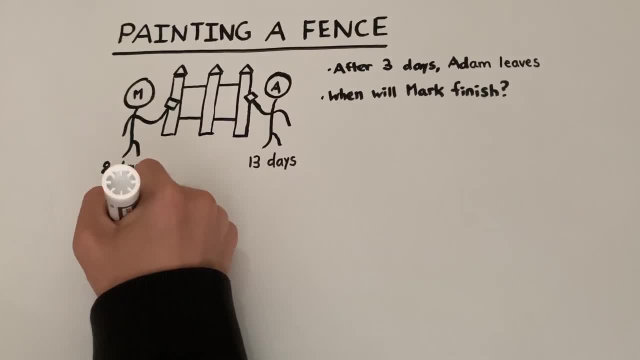 1 eighth of a fence. Similarly, Adam takes 13 days to paint a fence. that means in one day Adam paints 1 13th of the fence. Now, since these two are working together, that means in one day both of them. 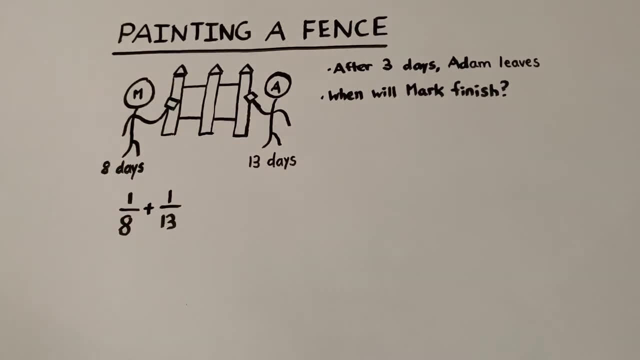 can paint 1 over 8 plus 1 over 13 of a fence. Now this turns out to be 21 over 104 of the fence that is painted in one day when Mark and Adam paint together. So after three days Mark and Adam have painted 3 times. 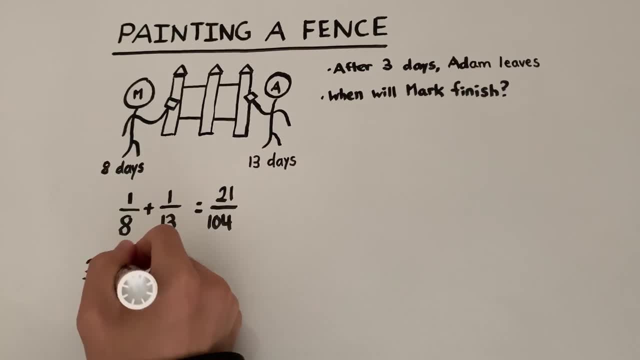 a fence 21 over 104, which is the same as 63 over 104 of a fence. So if this is how much of the fence is completed after three days of work, then when Adam leaves he is leaving 41 over 104 of the fence for Mark. 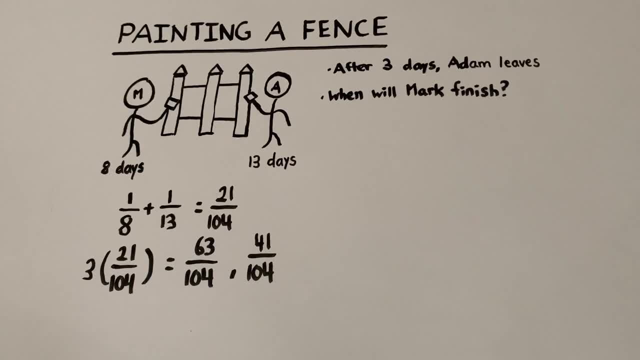 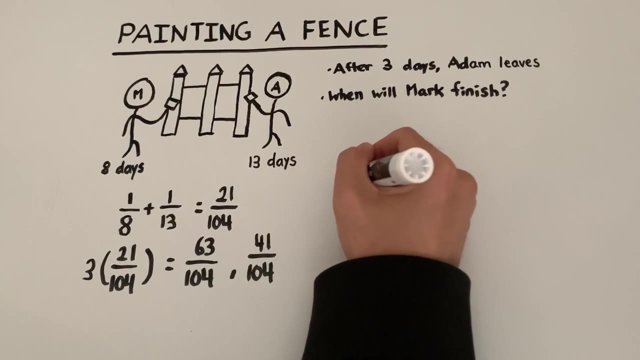 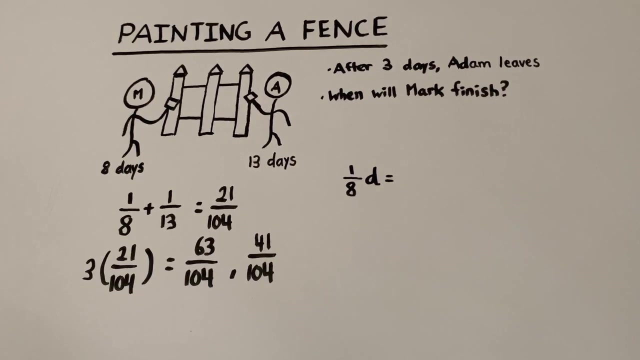 So now let's let D be the number of days that Mark paints alone. Since Mark does 1, 8th of the job every day, then we have 1 over 8 times D equals the amount of work left to be painted, which is 41 over 104..